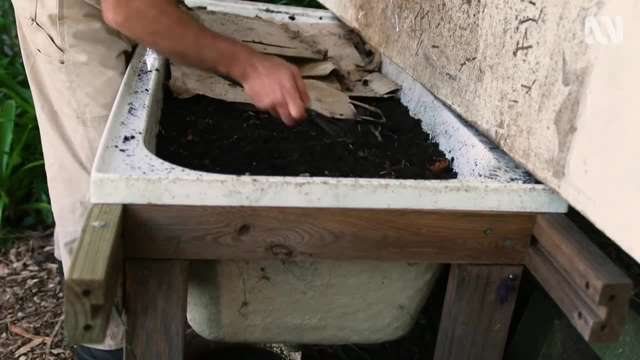 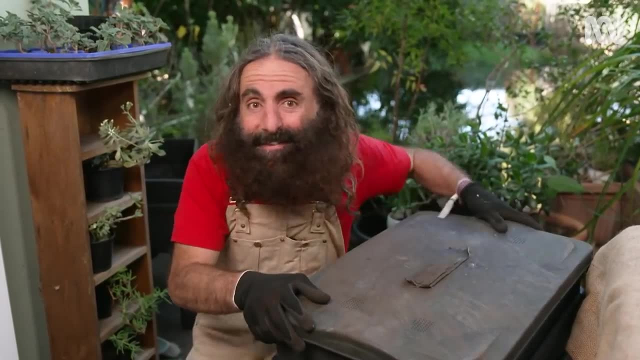 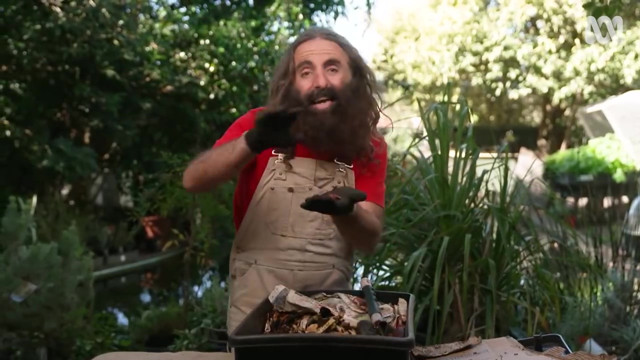 a whole bathtub and build a frame for it. The main thing from a location point of view is keep them out of direct sunlight or strong prevailing winds. The worms we use in farms are species that live typically in the top layers of the soil or the leaf litter, and they help to break down. 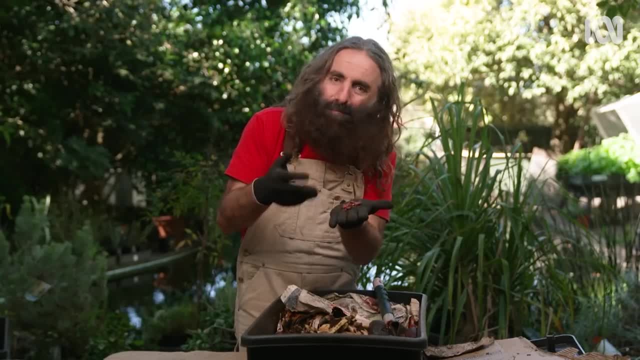 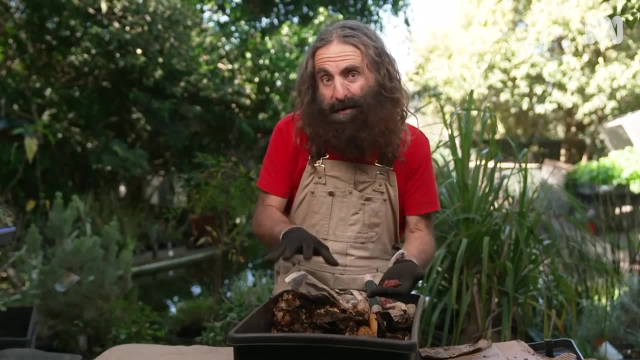 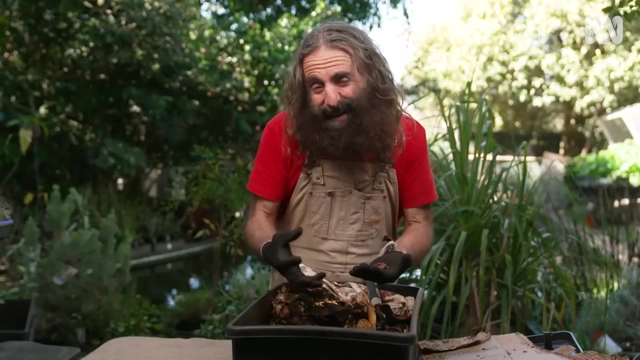 organic matter. Your farm needs to mimic this natural environment. Your worms need ample moisture and oxygen because they breathe through their skin. So this feeding layer, or call it the dining room, doesn't want to be saturated. It just needs to have a consistency of, say, a moist sponge. 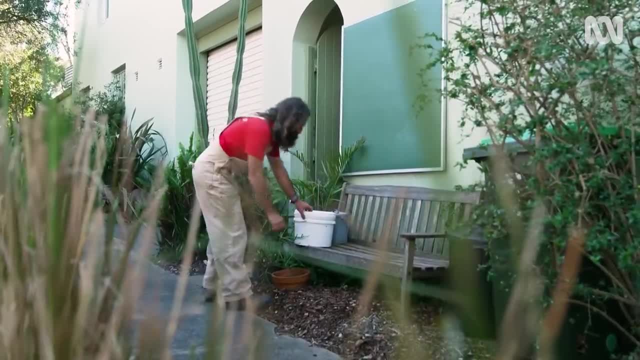 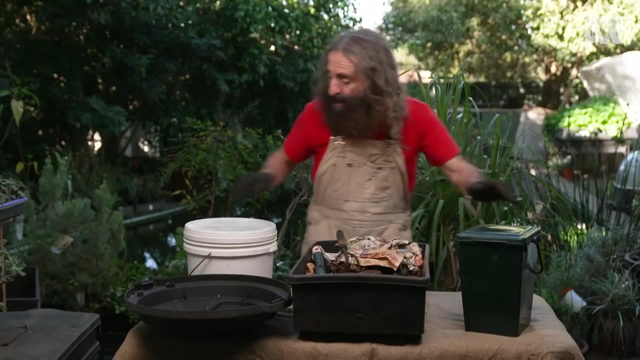 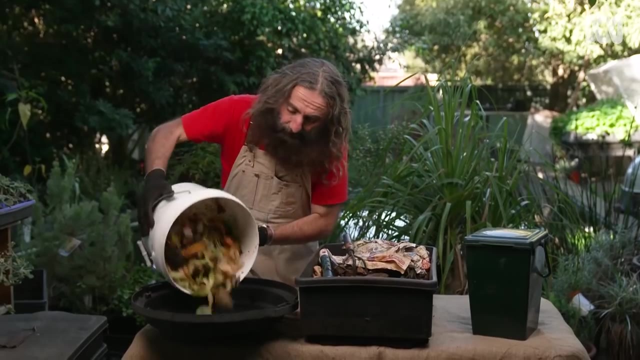 I'm lucky because I've got a plentiful supply of food scraps. There's my own that I put in my bench top tidy, but I also have my own little share waste system where about 15 houses bring me their food scraps and they drop it into this bucket and there's all sorts of different. 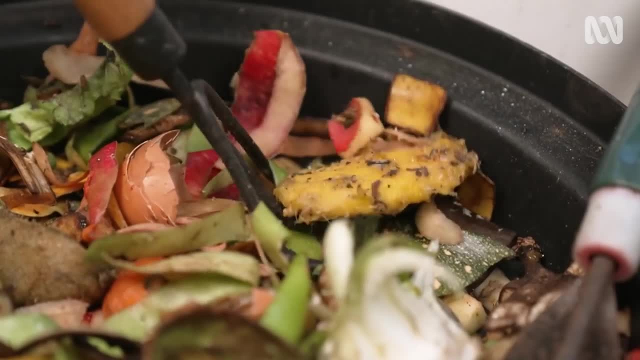 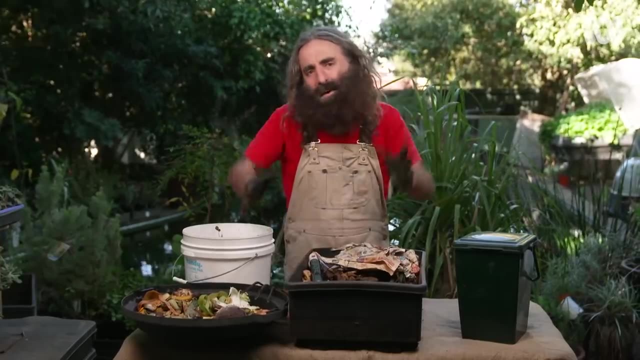 things that people include in these scraps. And the big question still remains: what can and what can't I feed my worms? Well, the key thing is diversity. You don't want all of the one same thing, Because this is- It's a living, breathing thing. 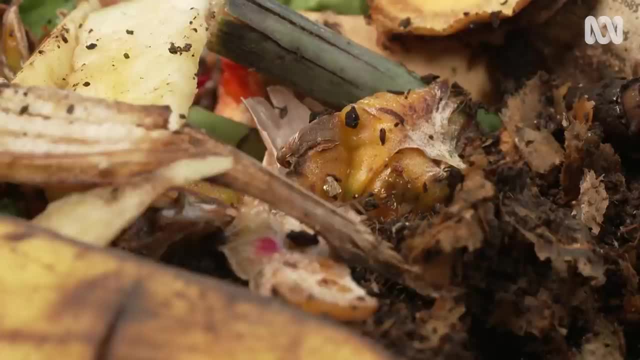 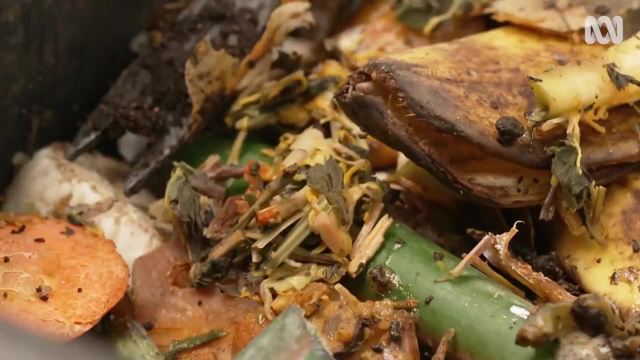 You don't want it to compact and block out all the air. I'm always asked: can you put citrus in a worm farm? The answer is yes, you can, but not too much, And the other thing you can do is actually put your citrus into the freezer. 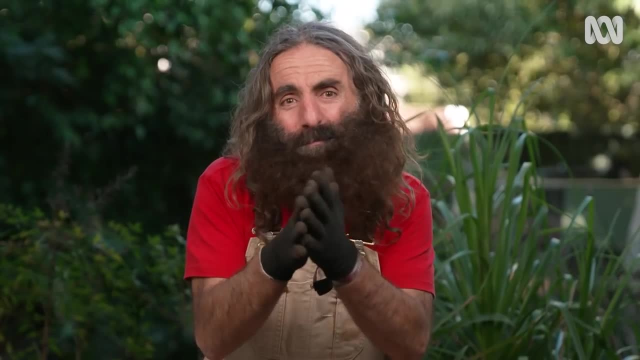 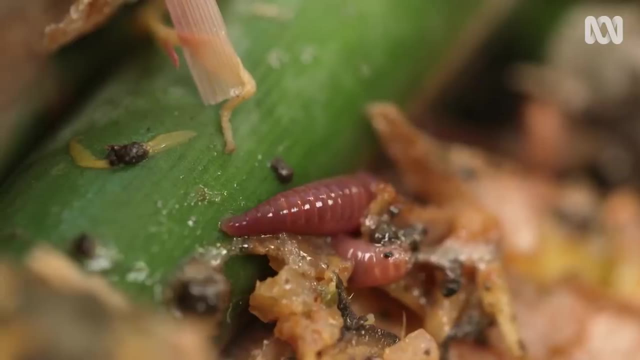 and when it thaws out and goes into the worm farm, all the cells have been broken by freezing and that way it's easier for the worms to digest it. Bear in mind that you don't want to overload your worm farm with too many scraps. Put enough out and then monitor it, and as you get a feeling for how much and how long it takes for them to eat what you put out, you can then add more as your worm numbers increase. It's important to remember that worms only have small mouths. 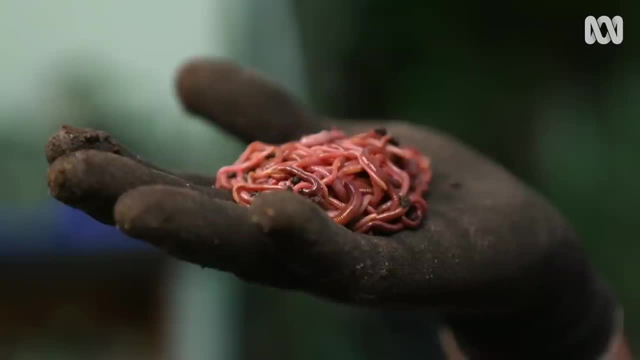 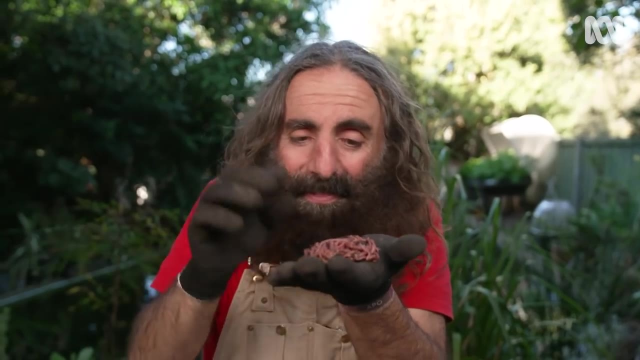 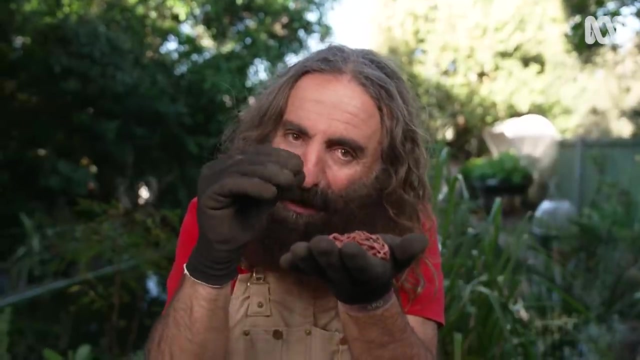 so they can't get themselves around really big chunks of food. When you're actually chopping up scraps, chop them a little bit more and then that way it'll be easier, but most of all quicker, for the worms to digest it. The other thing to remember is worms don't actually have teeth. 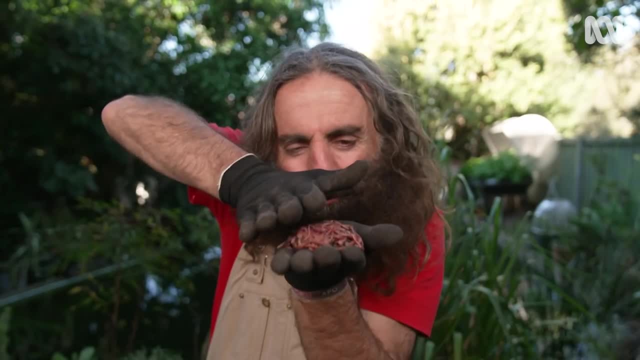 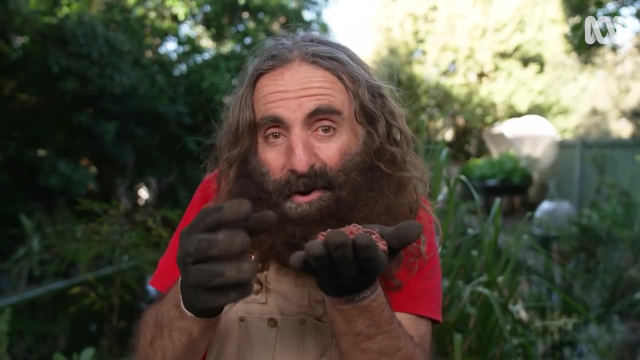 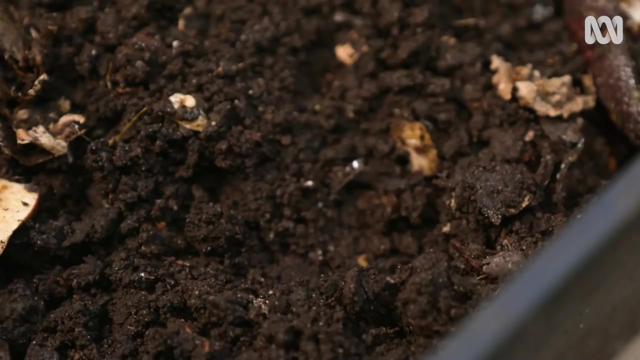 What they do to break food down is grind it through their stomach. and to help in that grinding process, a little scoop of garden soil from time to time will add some grit, and that grit helps crush the food and turn it into castings a lot quicker. 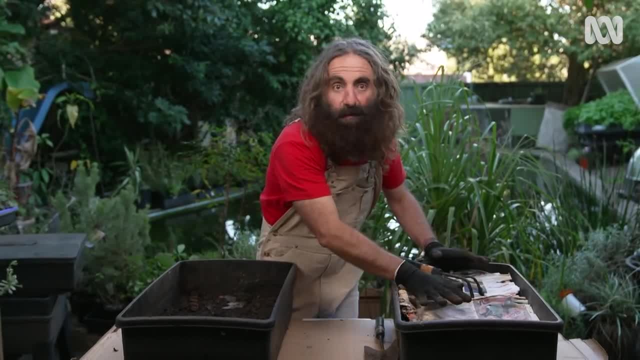 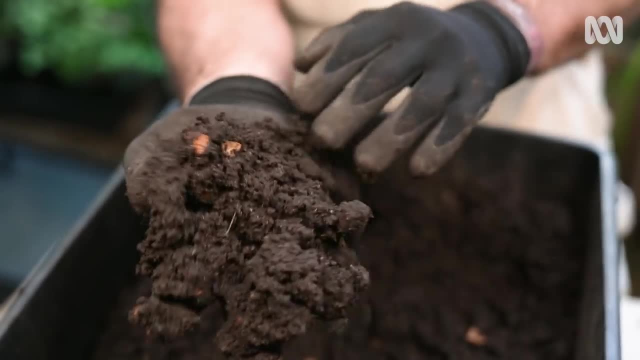 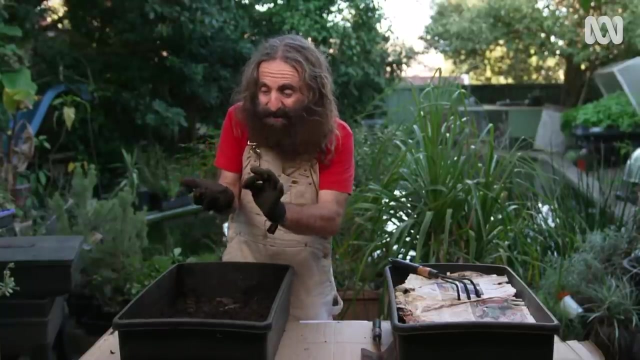 Now, when your worm farm here is full and the worms have eaten all the scraps, what you end up with is this, which is this beautiful rich worm castings, otherwise known as worm poo, because they've digested it and turned it into this fertiliser for your garden. 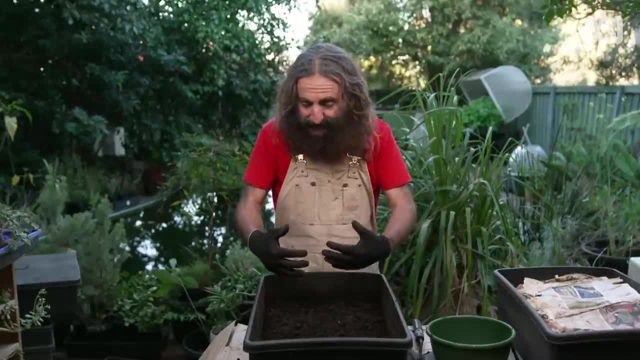 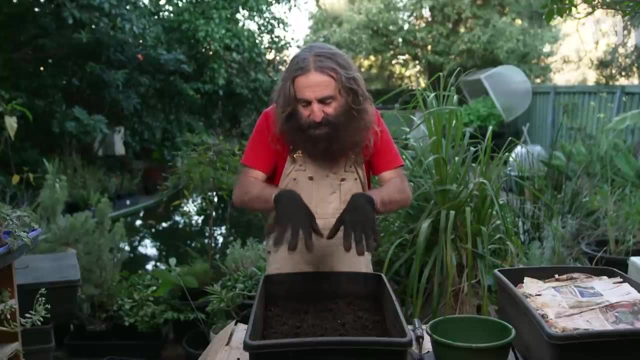 Now, besides that, there's also a lot of other things that you can do. The simplest method that I find for harvesting the worm castings is to start to scrape layers off and give the worms a chance to dive down out of the light. 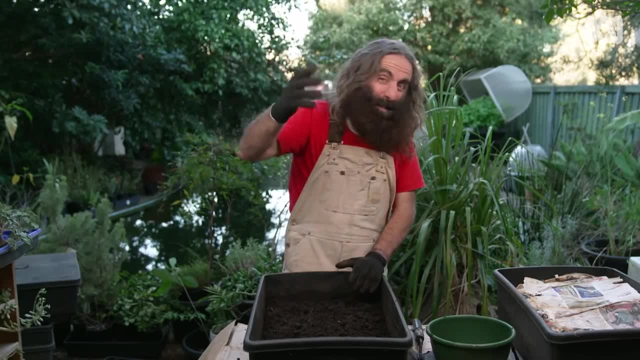 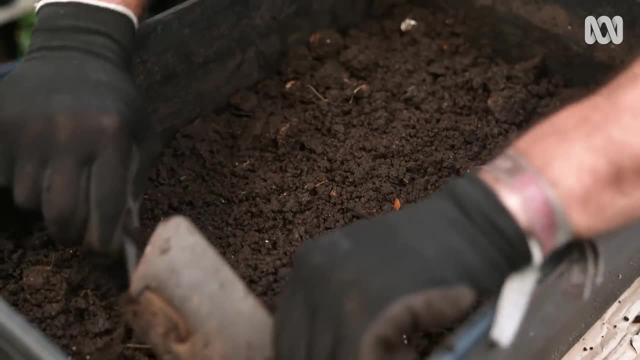 just like teenagers: if you open the curtains early in the morning, They don't want it. They hide under the doona and go deeper and deeper. So what I like to do is take off the first couple of centimetres, because in that layer there's usually eggs and babies. So what I like to do is take off the first couple of centimetres, because in that layer there's usually eggs and babies. So what I like to do is take off the first couple of centimetres. so I want to save those. 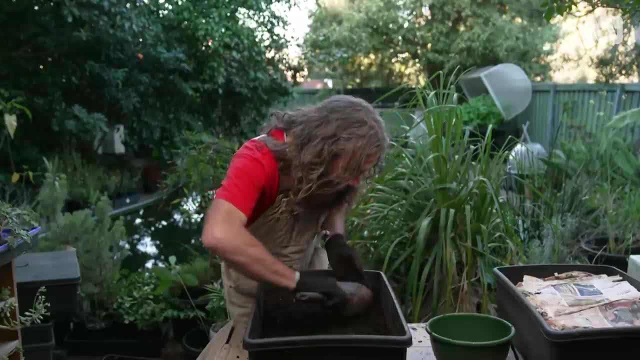 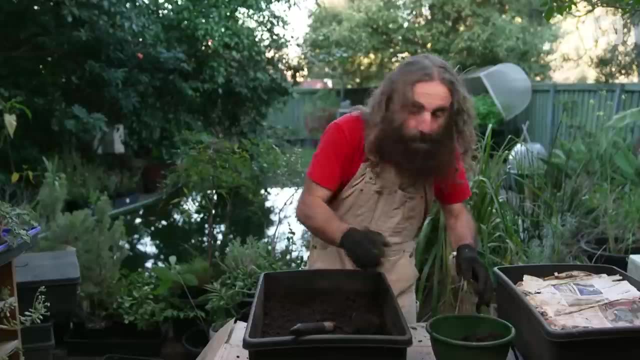 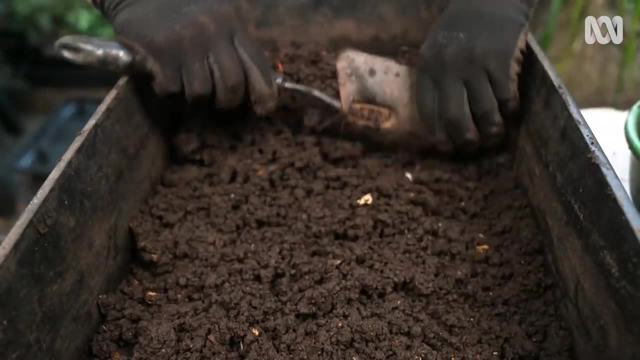 So I just scrape that off like so, and I put it aside into a separate container and I'll put that back in at the end. Next I start to scrape down around about 20 millimetres, And as I scrape I just keep an eye out. 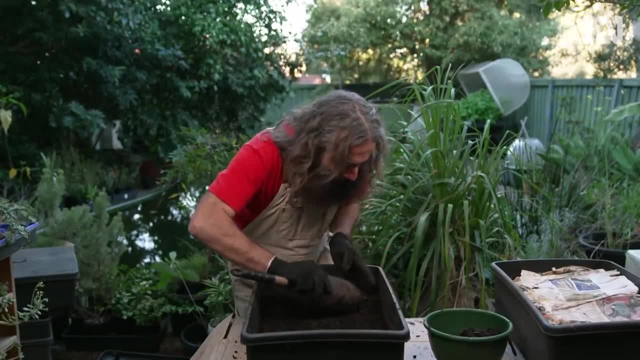 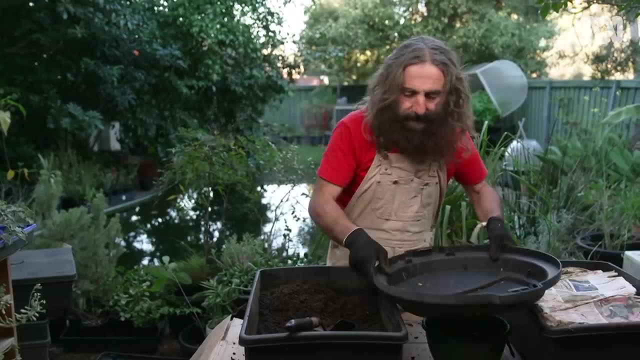 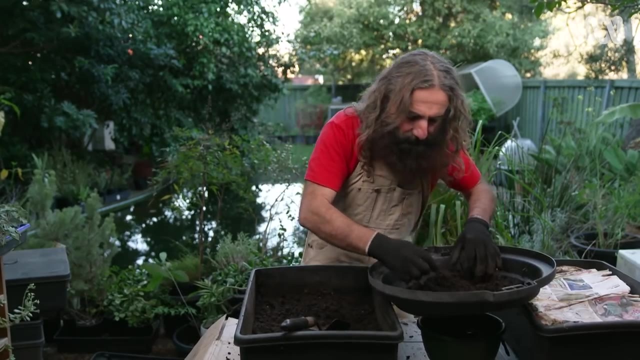 and see whether I'm coming across any worms. But at this point I can't see any, which is good. So I've got another container here and I'll just pick that out And look: there's one worm. If you see one, just save it, put it in there. 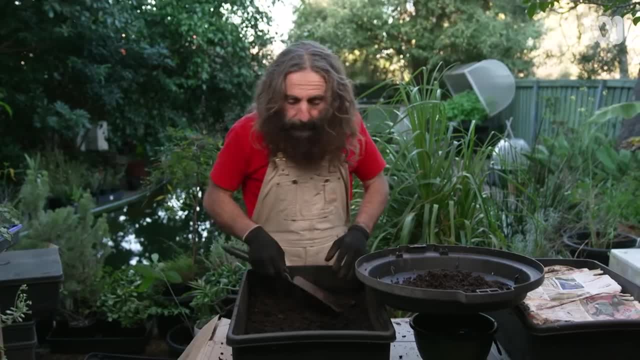 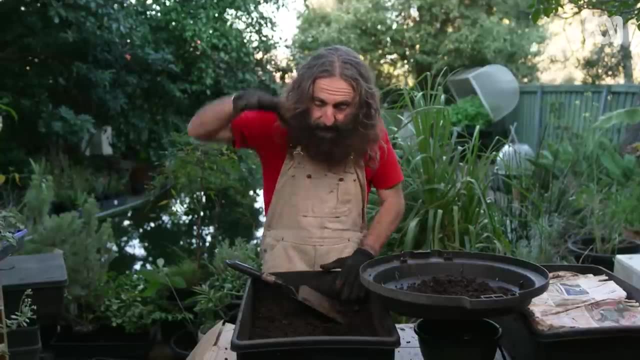 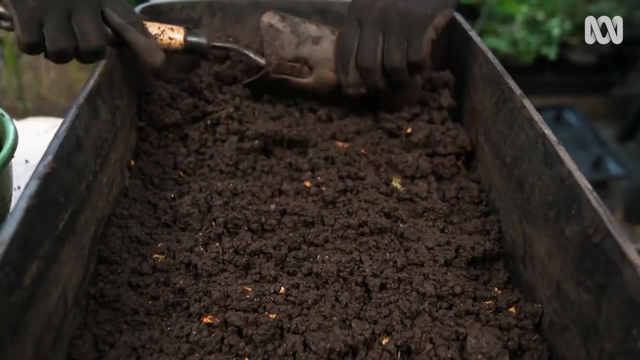 That's fine. And now normally I'd wait about 10 minutes and that way the light beaming down on here is forcing the worms further south. Then we go again. Once I reach pretty close to the bottom, or where there's a lot of worms, I say: